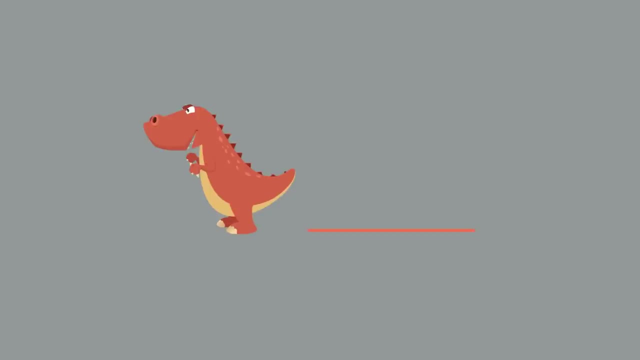 odd This dinosaurs all alone. He's not a group of 2.. This makes the number one an odd number because he's alone. That's odd. It's an odd number. Let's look back at the number two. Let's look back at the number two. See what's. 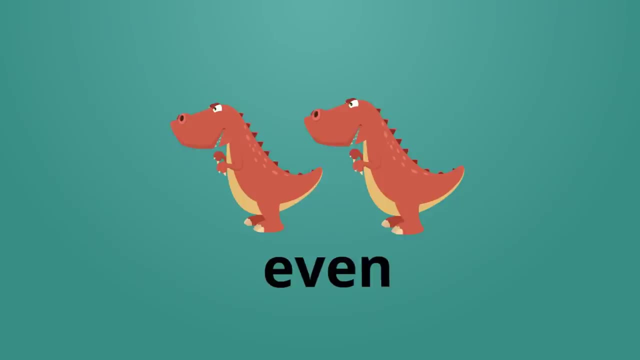 See what's neat about it. Here is the key switch. You're looking for the number 2.. You're about this is it's an even group of two? That means our dinosaur has a friend. He can talk to his friend, He can hang out. It's not weird, It's not odd, It's an even number. Here we 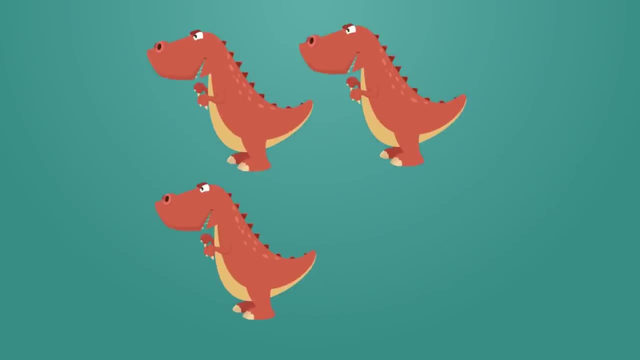 have three dinosaurs Now can we put the number three in even groups of two? Well, no, because that third dinosaur is all alone. The top two dinosaurs have somebody. Three is odd. There's one that's missing a partner Here. we have four dinosaurs. Now we're looking. 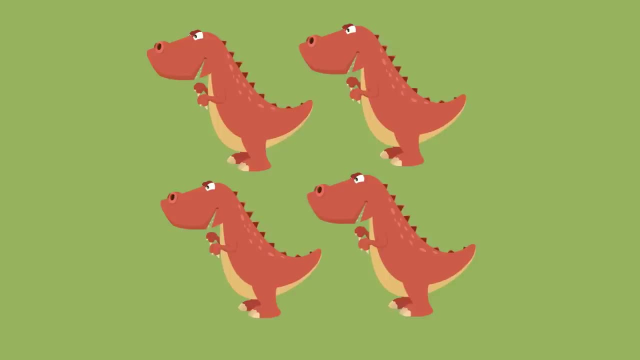 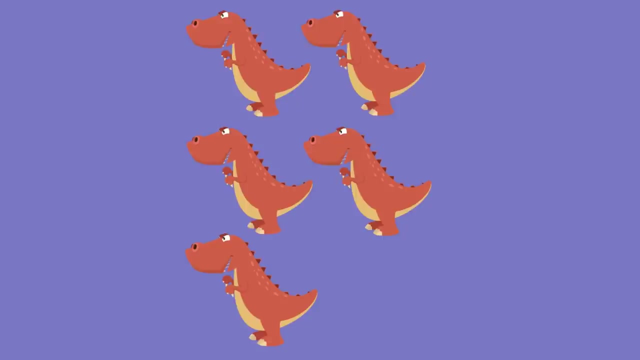 for groups of the number two. Now we have two groups of two here. That means it's an even number. Each dinosaur has a friend. Wow, Five dinosaurs. But look, One on the bottom doesn't have a pal, doesn't have a friend. That's odd. It's not evenly grouped into two. 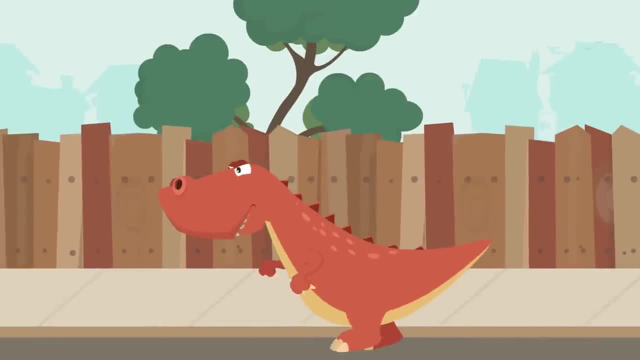 Five is an odd number. Hey, buddy. Okay, Don't don't run. Okay, We'll get back to the even numbers. I know you don't like the odds, You don't like being the odd dinosaur out. It's okay. 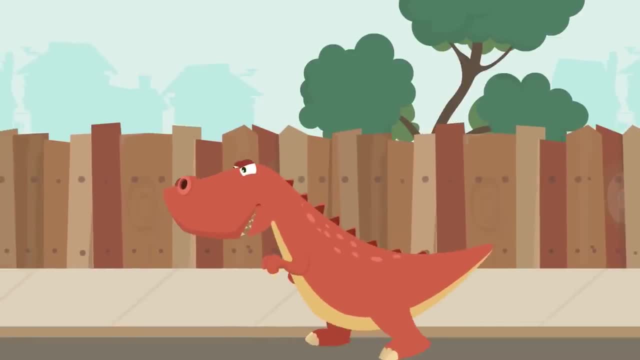 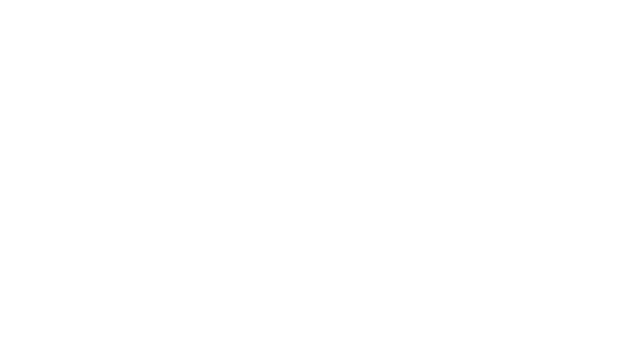 I promise this next number is going to be even, because it goes for even odd. even odd, Just hang on, Man, dinosaurs, you know, so temperamental I mean. what's that all about? I mean, a dog, dog wouldn't have done that, You know. dogs are better, I think, now, than dinosaurs, you know. 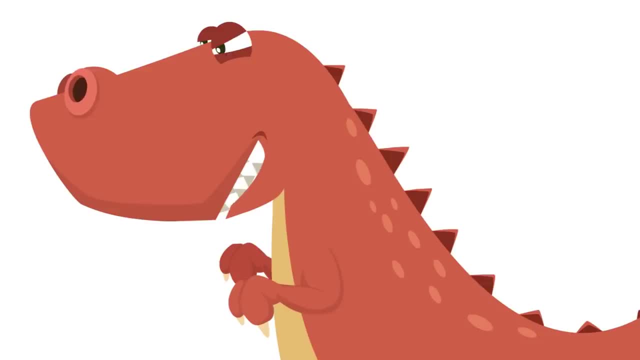 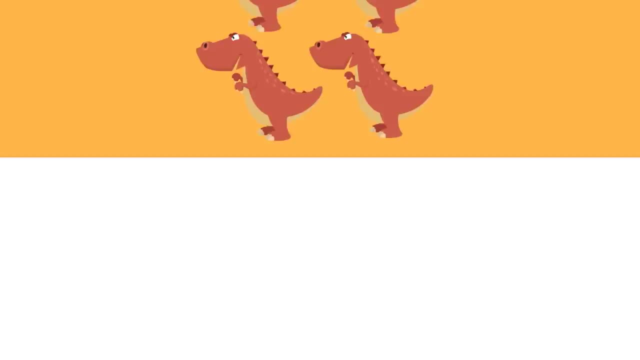 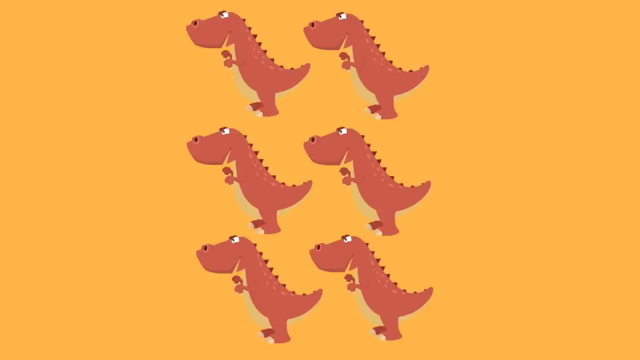 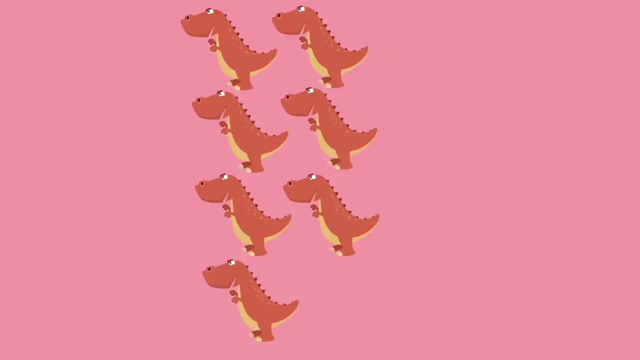 I'm just kidding. Dinosaurs are so cool Moving on. Here we have six dinosaurs Now each dinosaur has a friend. That means six is even. You can split it up in groups of two. Oh, here we have seven dinosaurs, but there's one dinosaur. that's all alone. Six of them have. 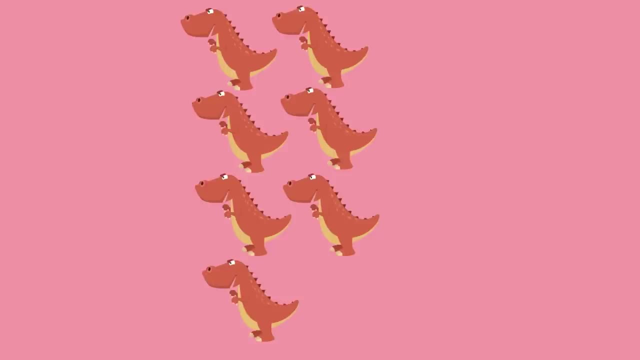 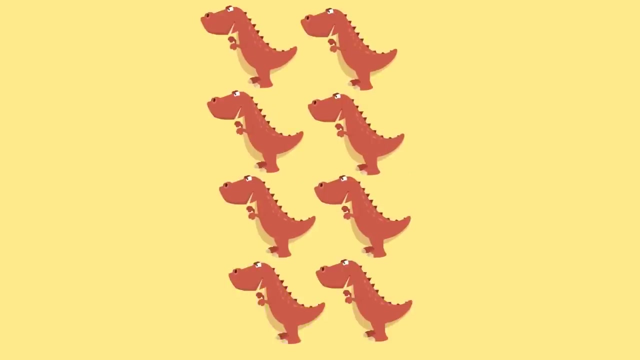 friends, but one is all alone. Doesn't have a pair. Seven is odd. The number eight: Does everyone have a friend? Yes, There's no one without a friend. Number eight is an even number. It splits up into two very nicely. Eight is even. 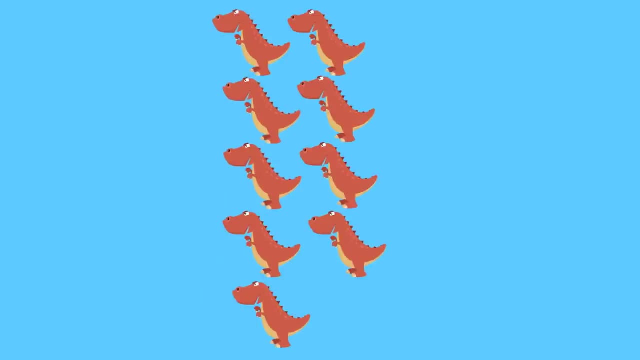 Let's go even higher. The number nine, Now you can see really quick, it's easy to spot. Is nine even or odd? Yes, it's odd. There's one who doesn't have a friend. Nine is odd. Oh, my goodness. Ten Ten, Is it even Or is it odd? You tell me, You know how to do it. 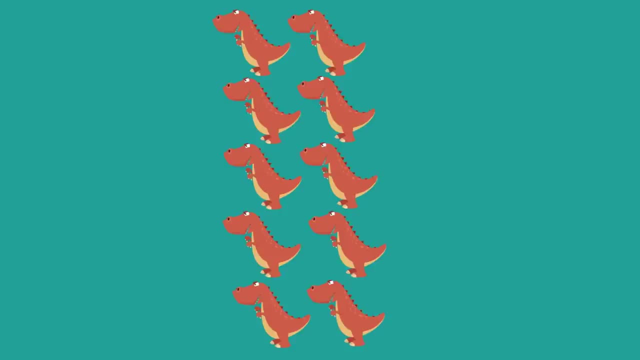 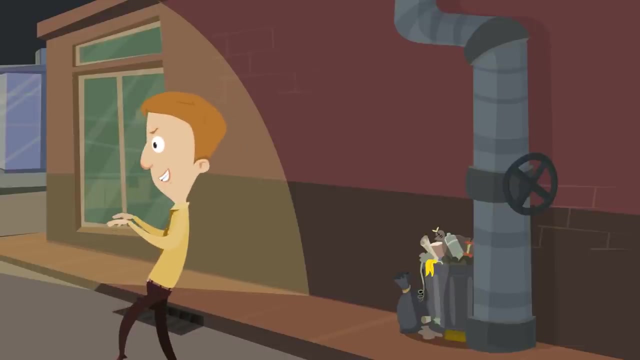 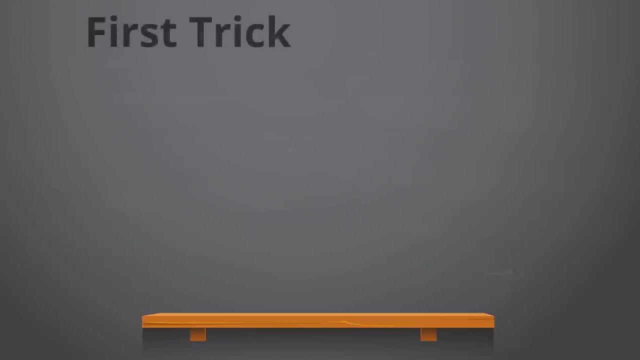 now You know the trick. Yes, Ten is even. Everybody has a friend. now we're about to teach you two sneaky tricks that you can use with even and odd numbers. okay, so seriously, it's well, it's okay, it's not. it's not really sneaky, but anyway. so this first trick. 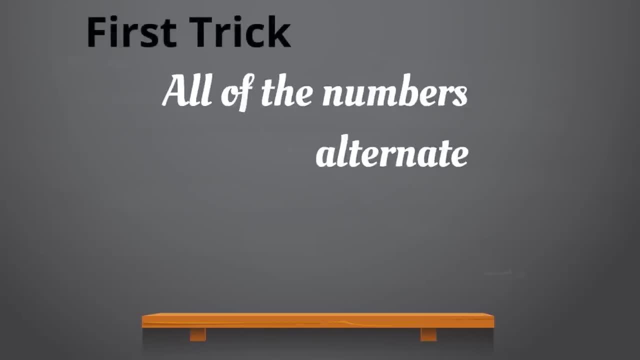 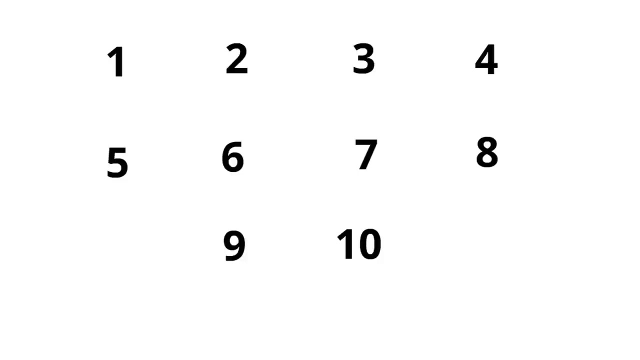 is that all of the numbers alternate from odd to even and back, and we're gonna show you what that means and what that looks like. here we have the first ten numbers, numbers one through ten, and the trick was: all of the numbers alternate from odd to even and back. do you remember if number 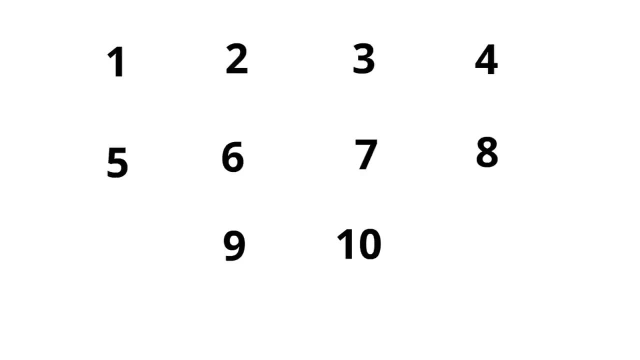 one is odd or even yes. number one is odd because, remember, number one's, all by himself, doesn't have a friend, doesn't have a partner. it's not an even number. number one is odd. now we remember number two, right. number two is even yes, because it can be. 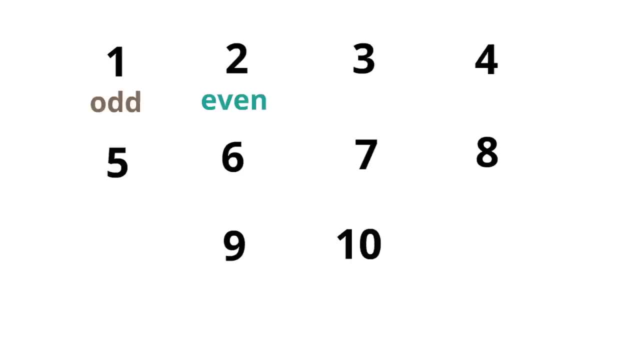 grouped in two because it is two. now, if they alternate, that means which one is number three? it's odd. this is where it gets fun. if three is odd, then that means four is even good job, and if four is even, that means five must be odd, yeah, and if five is odd, that means six must be. 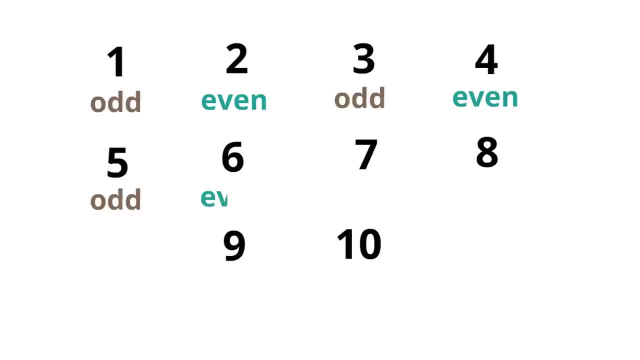 you guessed it, even. and if six is even, that means seven must be odd. yes, seven is odd. if seven is odd, that means eight is. come on, what's the pattern? eight is even. and if eight is even, that means nine must be odd. and if nine is. 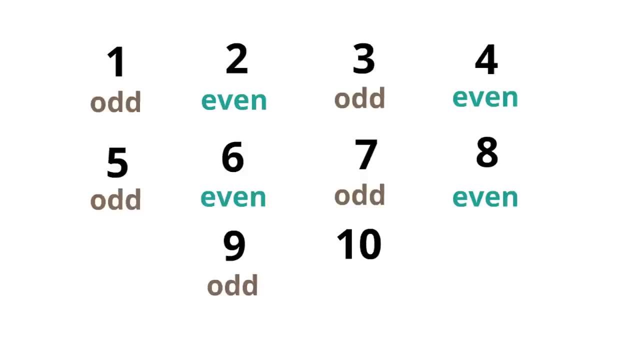 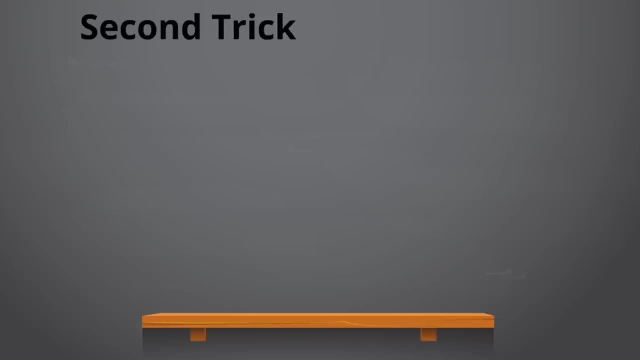 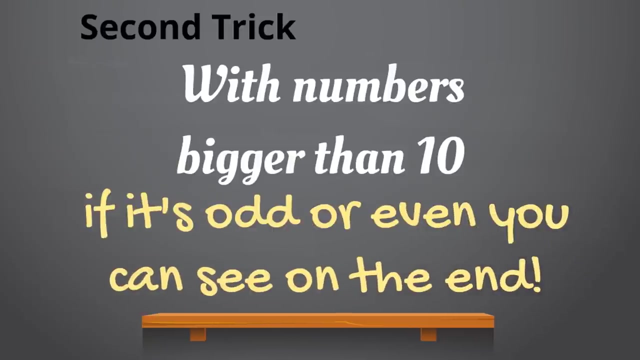 second trick is that with numbers bigger than 10 if it's odd, or even you can see on the end. with numbers bigger than 10 if it's odd, or even you can see on the end, to demonstrate. let's play a game we here at homeschool pop call odd or even. 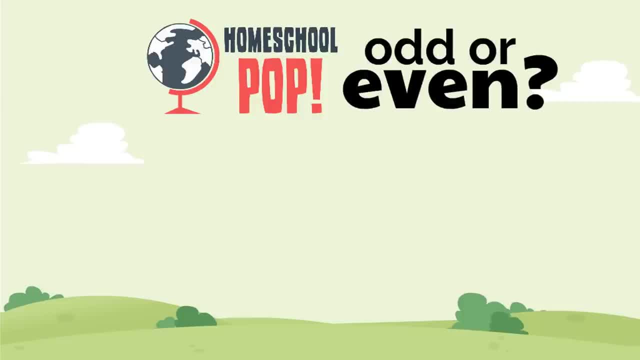 we're gonna look at a number that's bigger than 10. we're gonna look on the end to see if it's even or if it's odd. our first one is the number 21. is it odd or is it even? it's odd how? why will we look up? 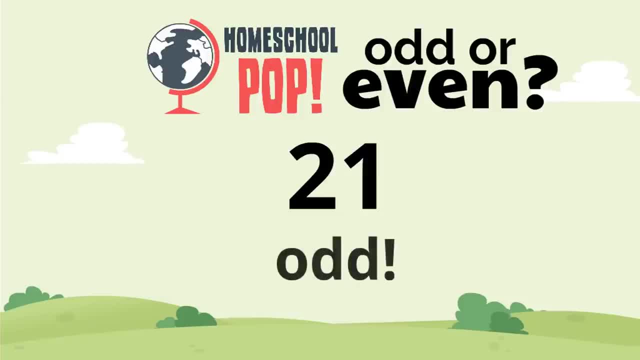 the end. the end is a 1. 1 is odd, it's all by itself a 1 is odd. so 21 is odd because 1 is the ending. did you know that means 71 is odd and 101 is odd and 131 is odd and the number 1001 is odd. why they all end in one. 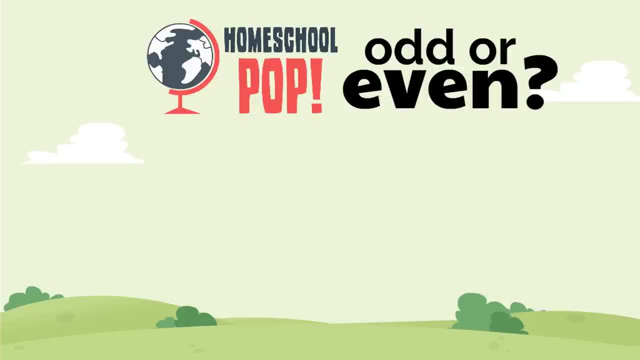 let's show you how to do that with numbers bigger than 10 and the number. try this one, the number 32. is it odd or is it even? 32 is even. well, how do we know? because of the ending. look at the ending. it's the number two. two is an. 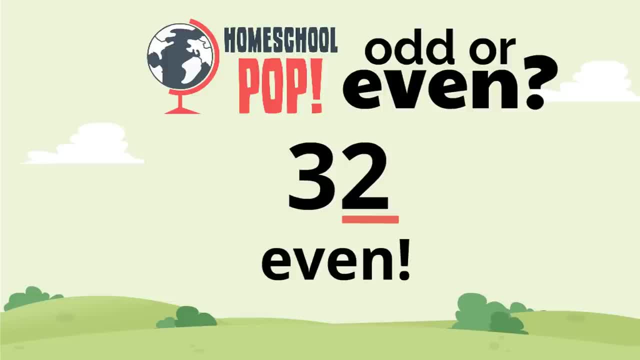 even number because it's a group of two. it can be put in groups of two because it is two. the same rule applies- this is the second trick- with numbers bigger than ten, if it's odd or even, you can see on the end every single number that 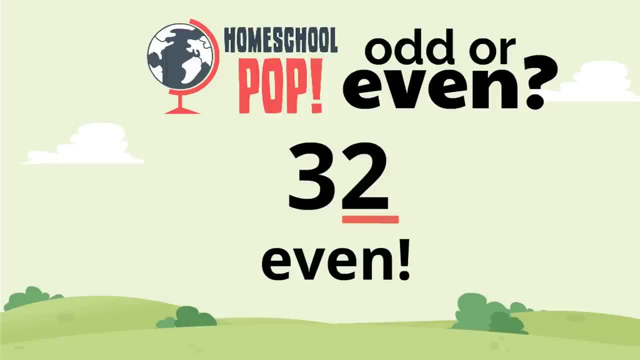 you can think of. ends in. two is an even number, let's try one. that's a little more tricky. let's try the number: 100 is 100 odd, or is it even even it's? 200 are even around 10, 20, 20, 30, 30, 30, 30 bored. oh, 100 is even it's. 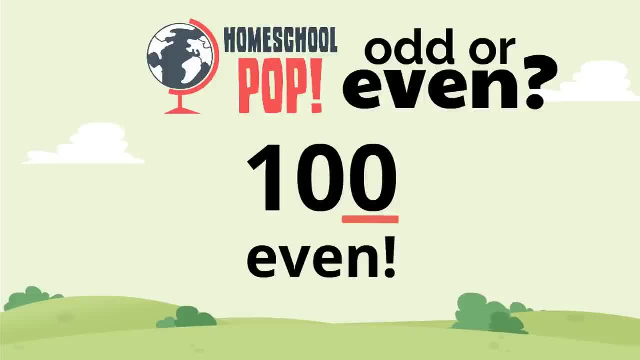 even, and we know that because of the ending, it ends in a zero. now remember. second trick: with numbers bigger than 10, if it's odd, or even you can see on the end, an ending is a 0 and every number that ends in 0 is even. let's look at the. 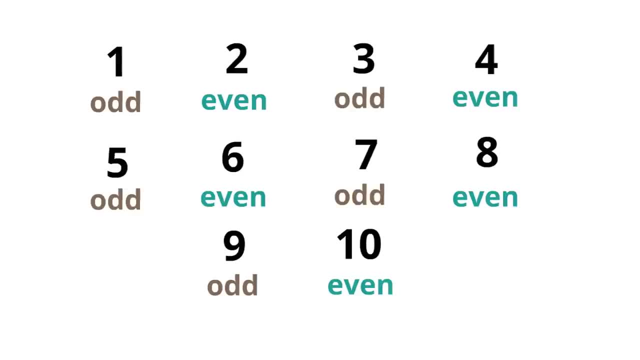 10 on the bottom ends in 0, and it's even. every single number that ends in a 0 is even. just like every number that ends in a 1 is odd, every number that ends in a 2 is even. every number that ends in a 3 is odd, because 3 is odd every number that